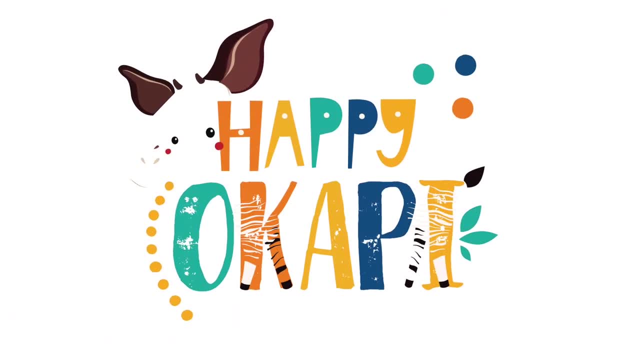 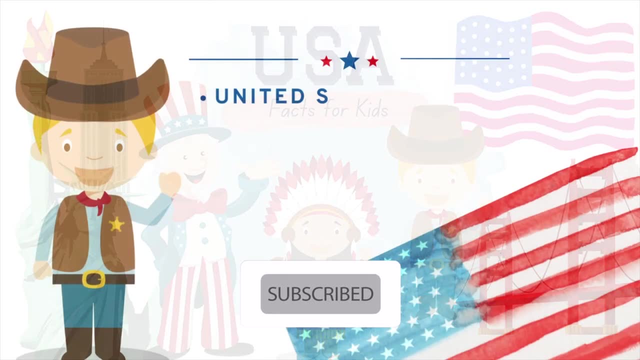 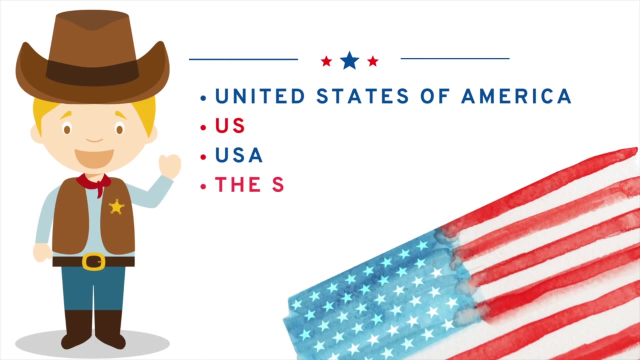 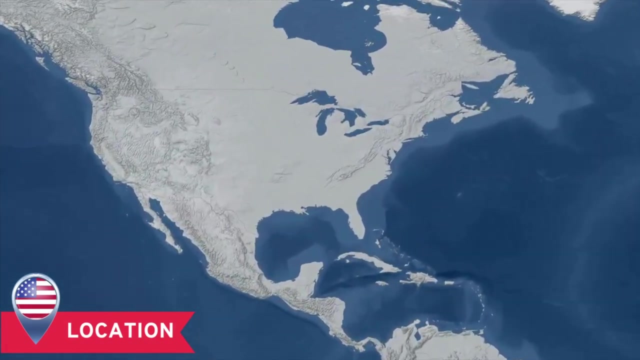 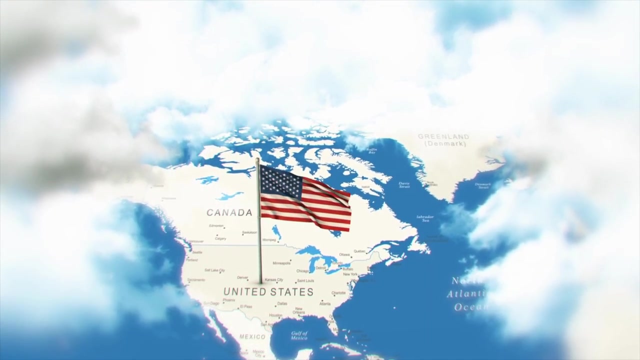 Hi everyone. Let's talk about the United States of America. It is also commonly known as US, USA, the States or America, even though America is the whole continent. United States is located in North America. It shares land borders with Canada on top and Mexico at the southern border. 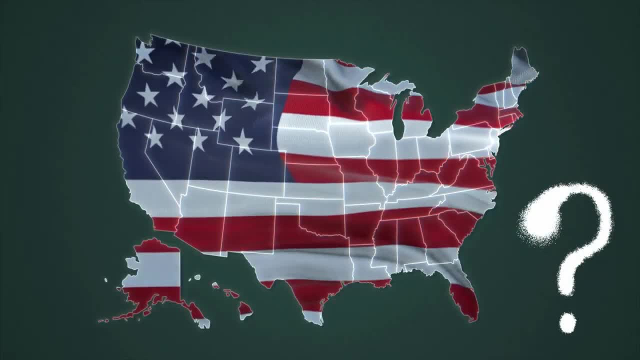 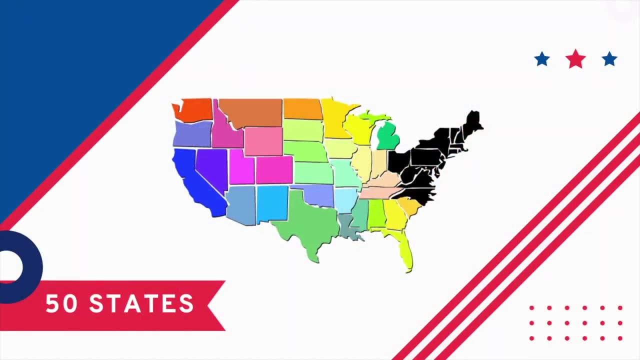 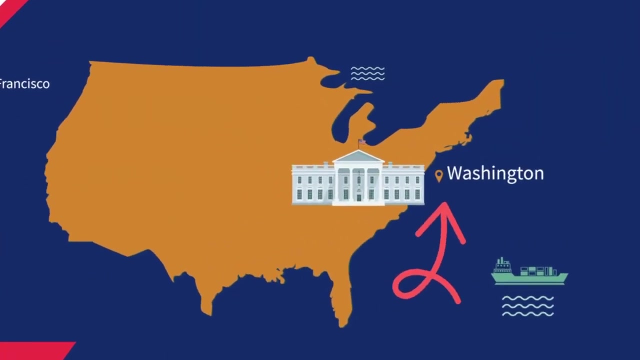 And do you know how many states does the US have? The US has 50 states. The 49 states, including Alaska, are located on the continent of North America, And Hawaii is located in the Pacific Ocean. The capital of the US is Washington DC And it is where the president lives. The president's house is called the White House. 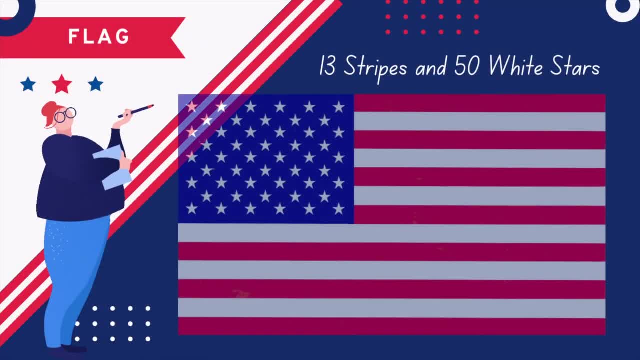 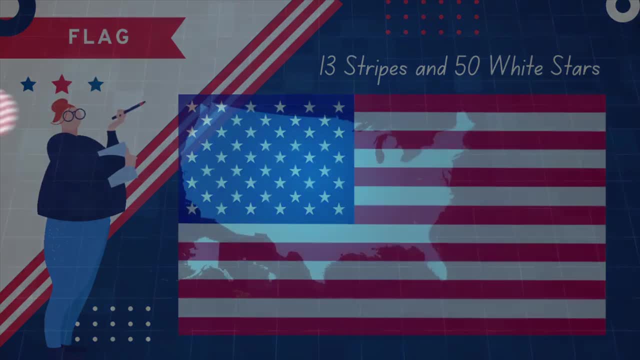 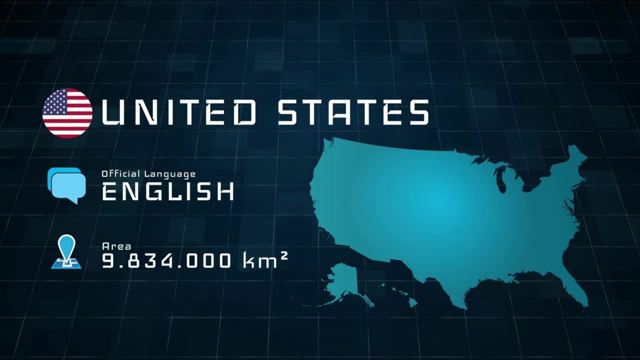 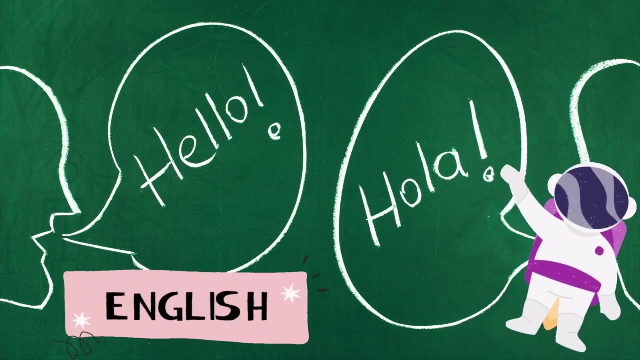 This is the national flag of the United States. It has 13 stripes and 50 white stars on a blue background. The most commonly used language is English, specifically American English, which is the national language spoken by the great majority of Americans. Many other languages are also spoken, especially Spanish. 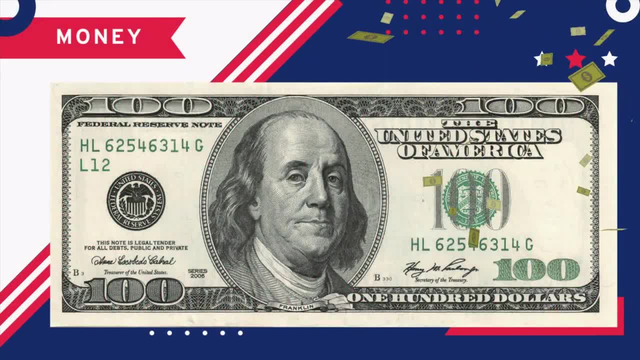 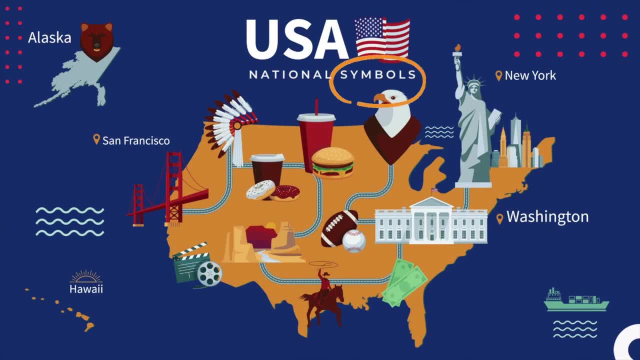 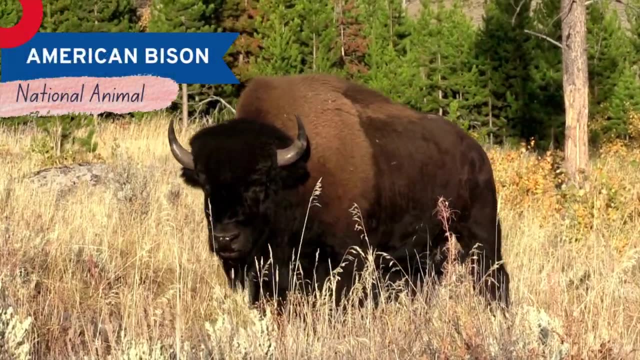 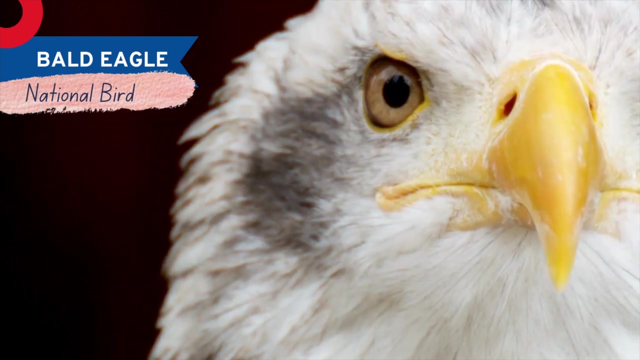 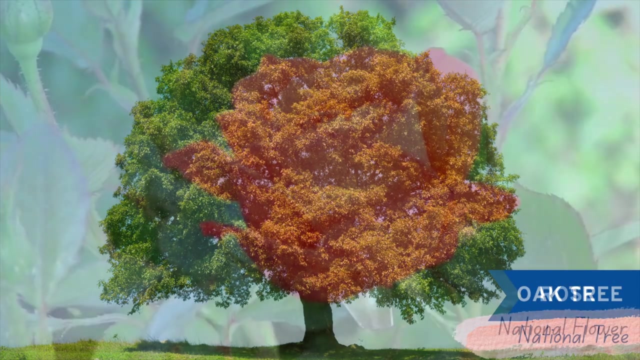 The money is the US dollar. Now let's see if you remember. what are the USA national symbols? The national animal is the American bison, The national bird is the bald eagle, The national tree is the oak tree And the national flower is the rose. 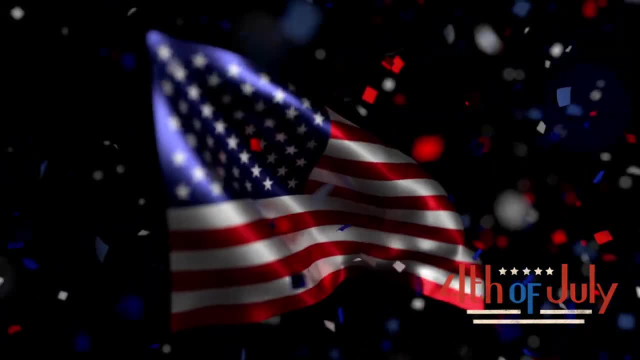 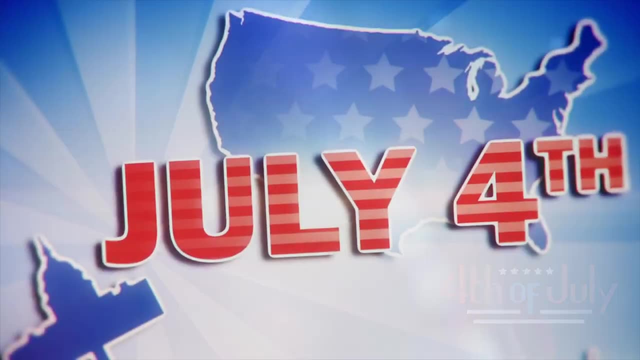 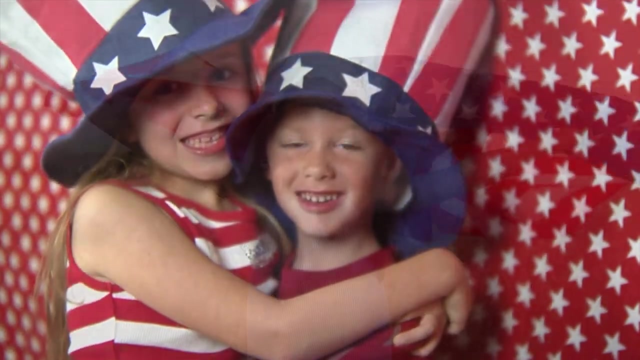 A very important date for Americans is the 4th of July, the national holiday of the United States, where they celebrate their independence on July 4th. Happy July 4th. Hot dogs and hamburgers are pretty traditional food for the 4th of July. 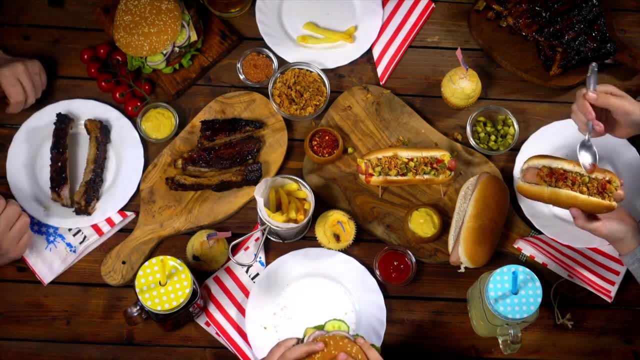 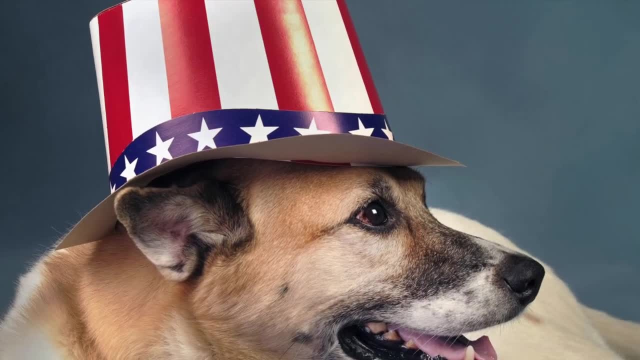 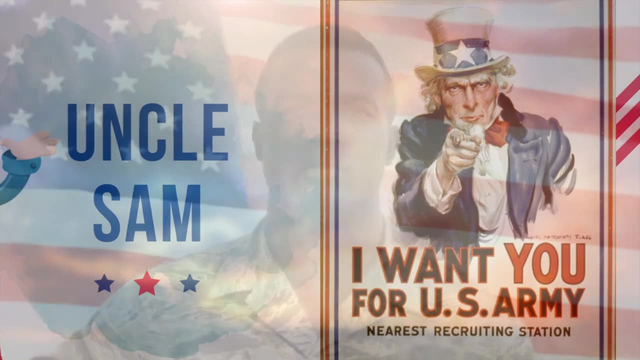 Now let's see if you can recognize this man. Probably you have seen him in t-shirts, posters, hats. Do you know his name? His name is Uncle Sam. This image was used to encourage men to enlist in the military service for World War I. 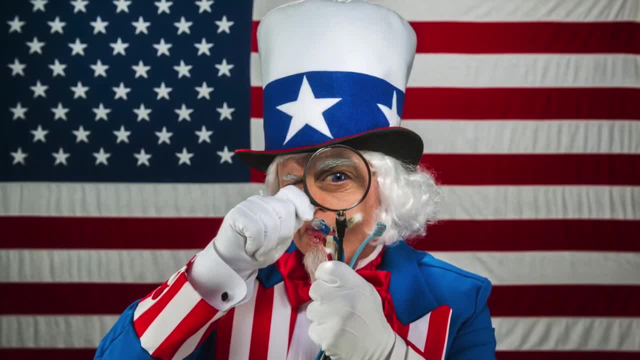 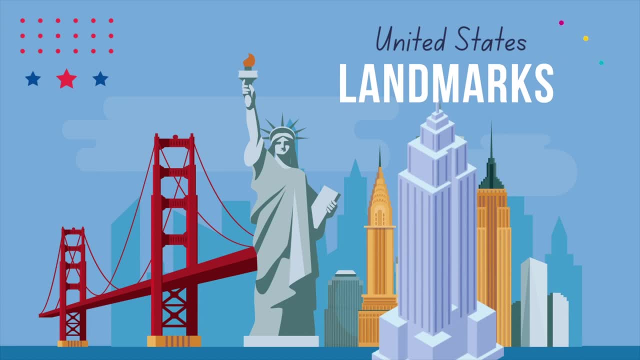 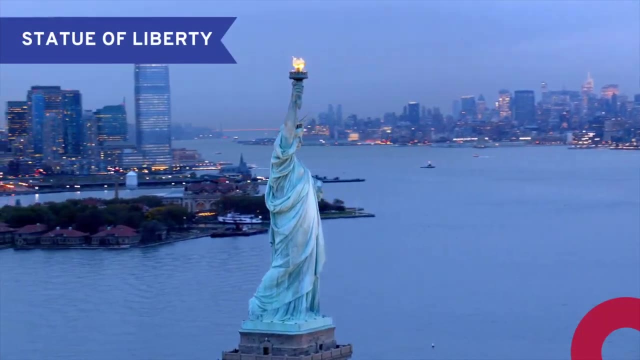 Uncle Sam was officially adopted as a military man. Uncle Sam was officially adopted as a national symbol of the United States. Now are you ready to travel to the US and get to know the most visited tourist sites and landmarks? The most famous one is a tall lady holding a torch. 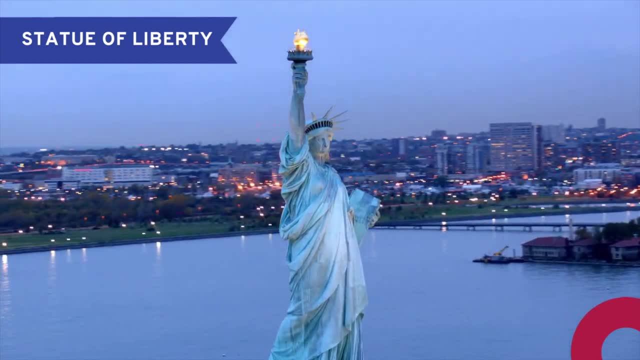 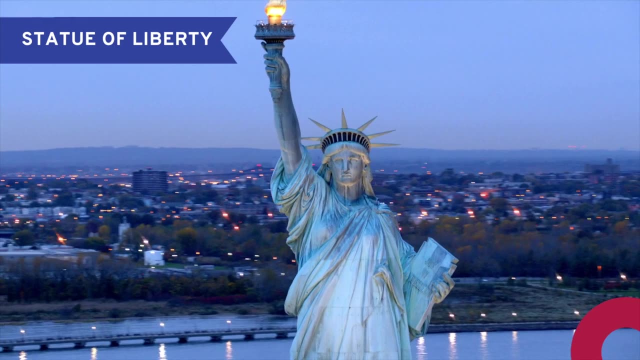 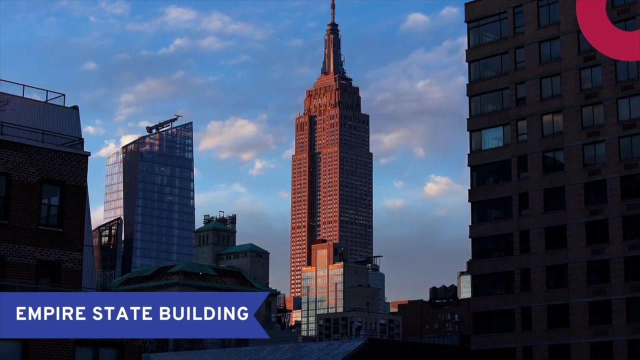 Do you know her name? It is the Statue of Liberty and it was a gift from France. It represents the freedom and liberty of the United States democracy. Also in New York, we can find the Empire State Building, one of the oldest buildings, which is over 100 stories high. 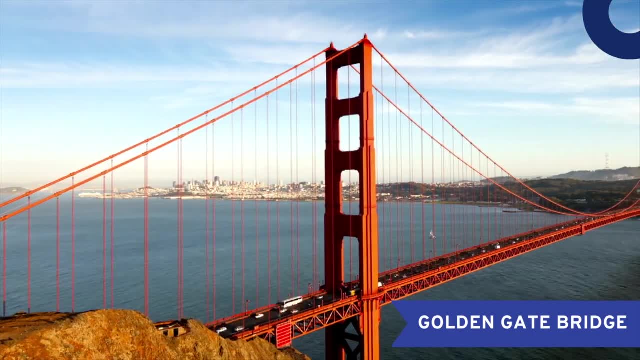 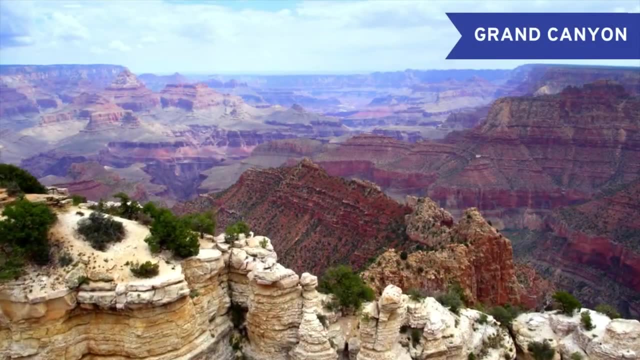 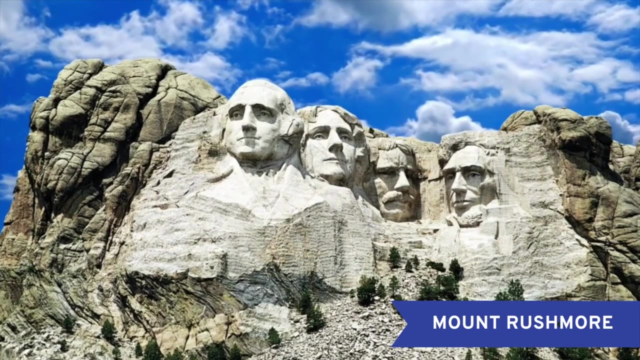 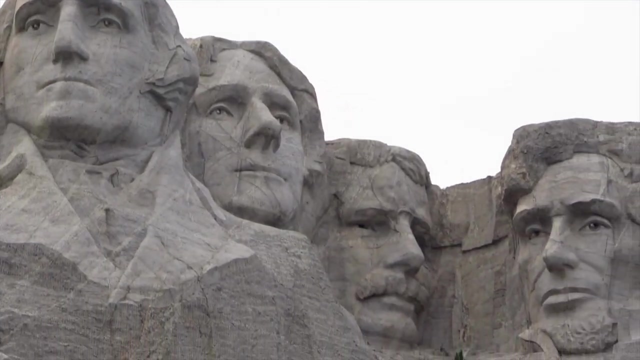 Then this famous red bridge is called the Golden Gate Bridge and it is located in San Francisco, California. Another important landmark is the Grand Canyon, located in Arizona. What about this mountain? Do you recognize it? It is called Mount Rushmore, and it is a mountain in South Dakota famous for the huge faces carved on its side. 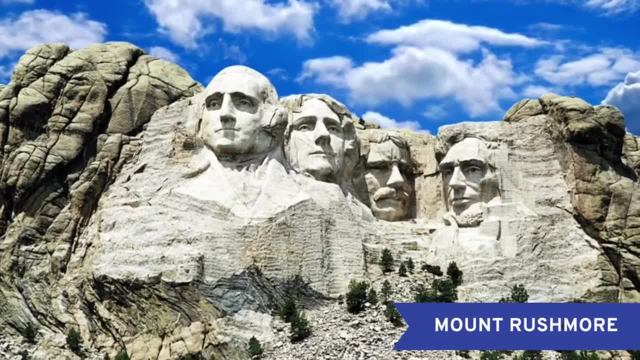 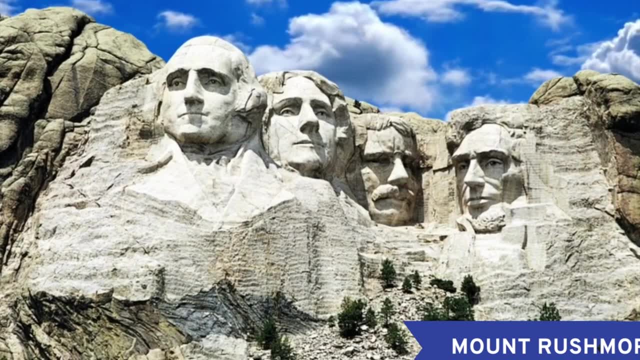 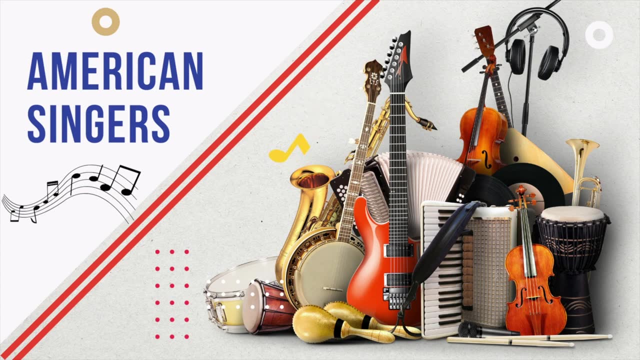 The faces are those of four US presidents: George Washington, Thomas Jefferson, Abraham Lincoln and Theodore Roosevelt. Now let's talk about music and sports. Not only the US is a huge country, But their musical impression has made a big impact on the world. 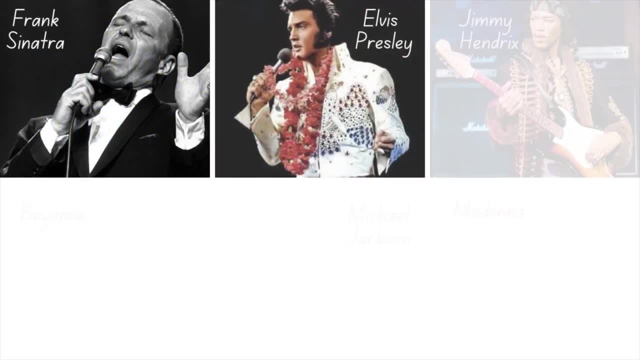 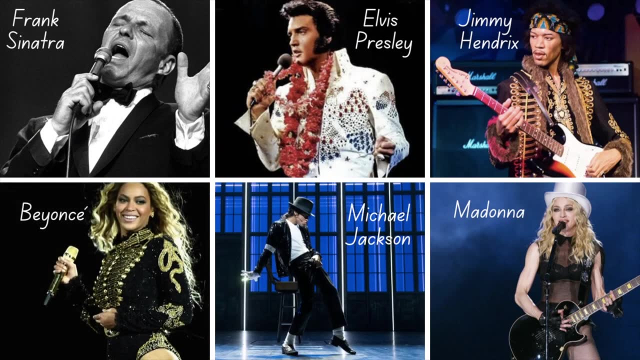 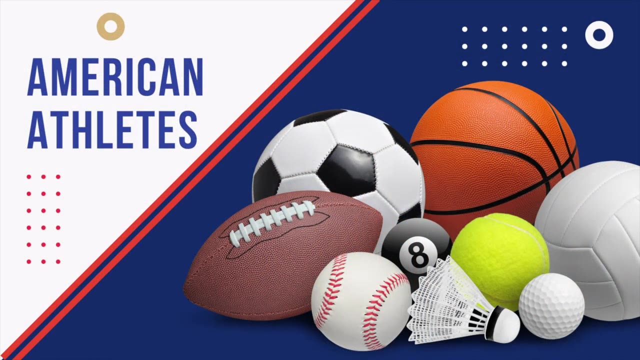 Some of the best musical artists include Frank Sinatra, Elvis Presley, Jimi Hendrix, Madonna, Michael Jackson, Beyonce and many more. And what about sports? The United States is a sport-minded country, with millions of fans who follow American football, baseball, basketball, tennis, golf and ice hockey.